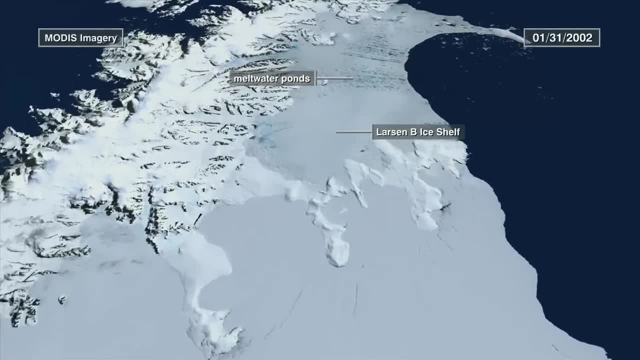 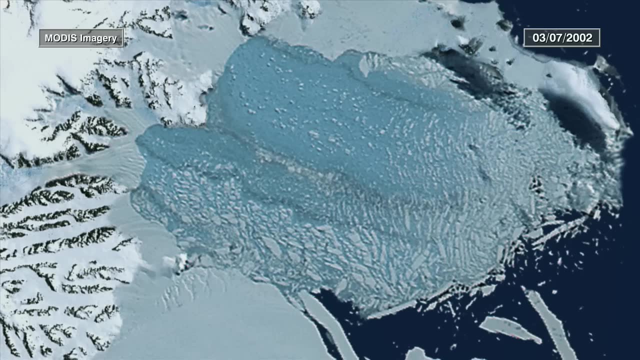 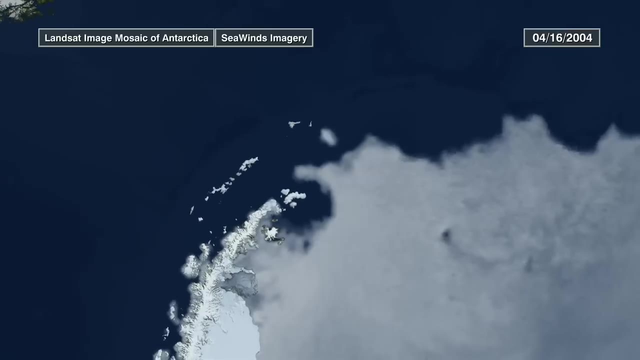 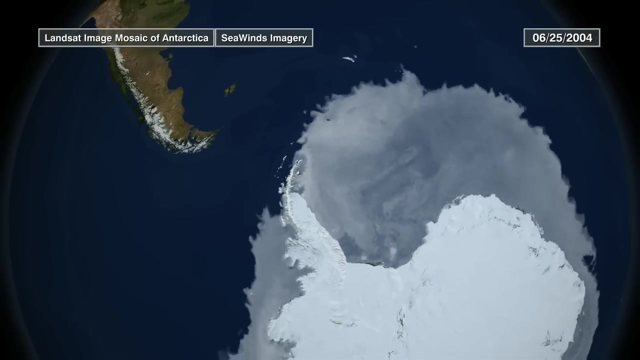 collapse. After 12,000 years, the Larsen B ice shelf collapsed in just five weeks. Offshore sea ice forms when the surface of the ocean freezes, pushing salt out of the ice. The cold, salty surface water starts to sink, pumping deeper water out of the way, powering 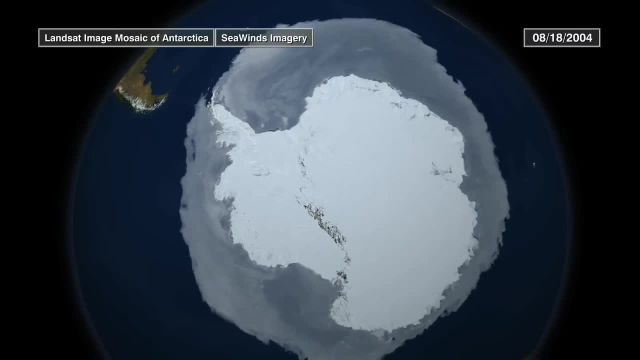 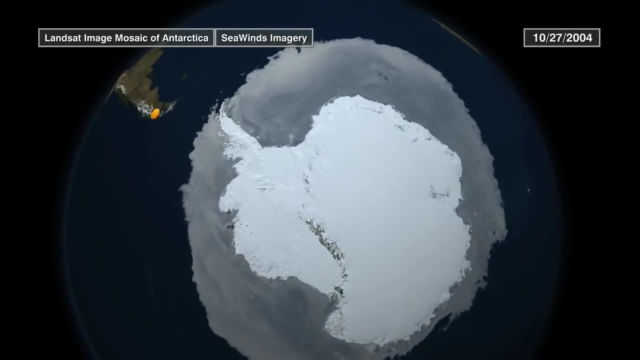 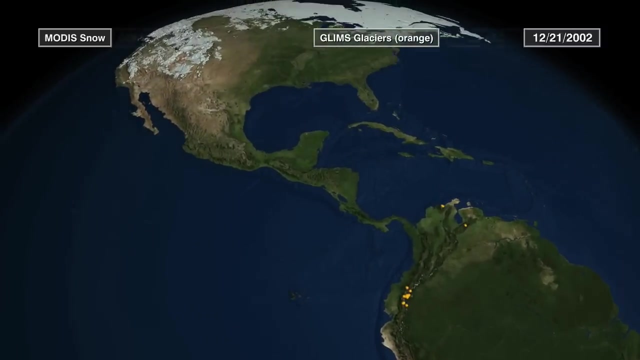 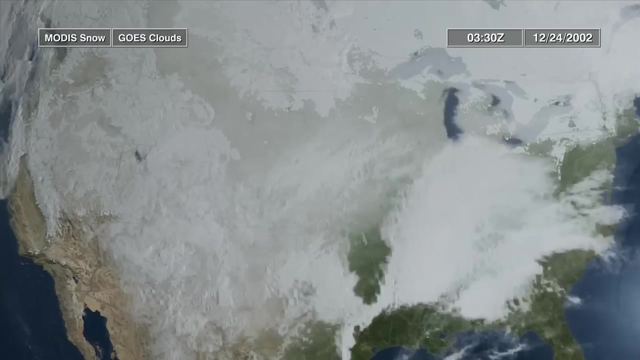 global ocean circulation. These currents influence climate worldwide. Most ice exists in the cold polar regions, but we see glaciers like these in the Andes all over the world. Most are shrinking. A tsunami, another one is coming Here in North America. millions of people experience the cryosphere every year. 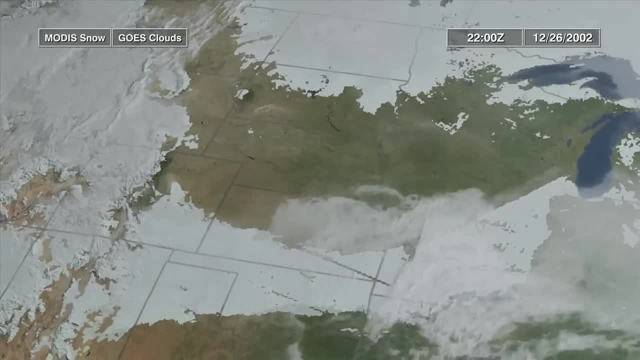 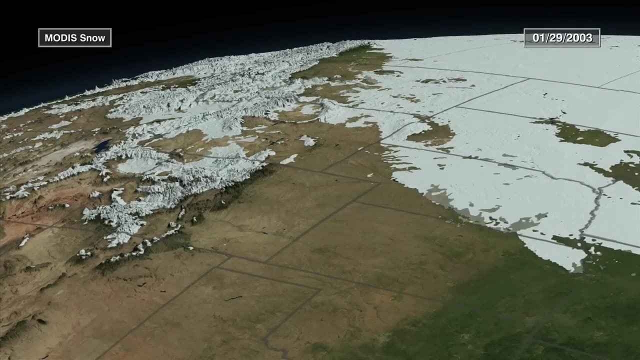 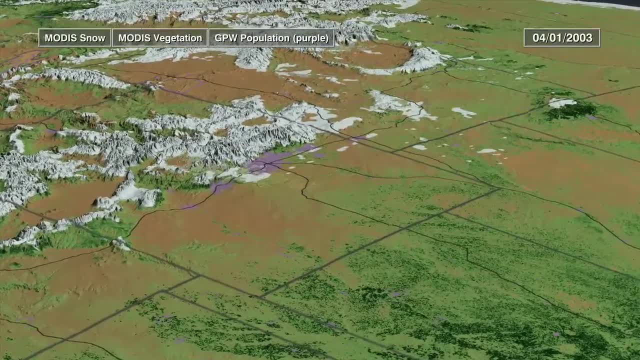 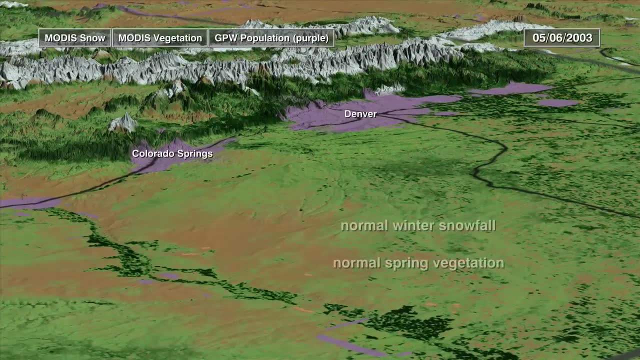 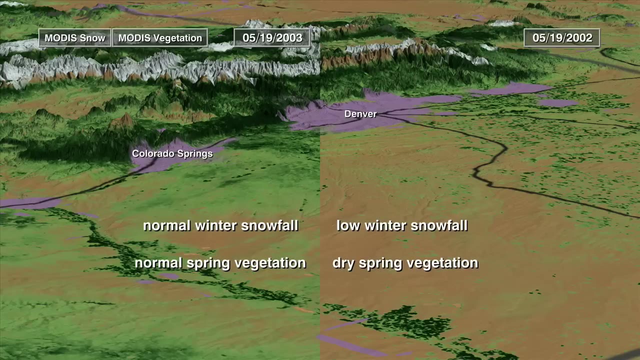 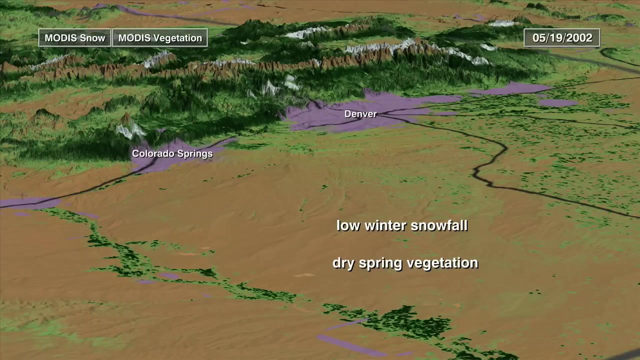 It's growing. Substantial winter snows produced a green Colorado in 2003,, but drier conditions the previous year limited vegetation growth and increased the risk of fires. In the Rocky Mountains there are patches of frozen ground, called permafrost, that never. 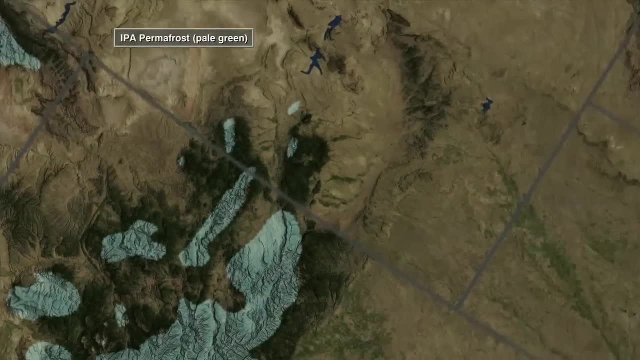 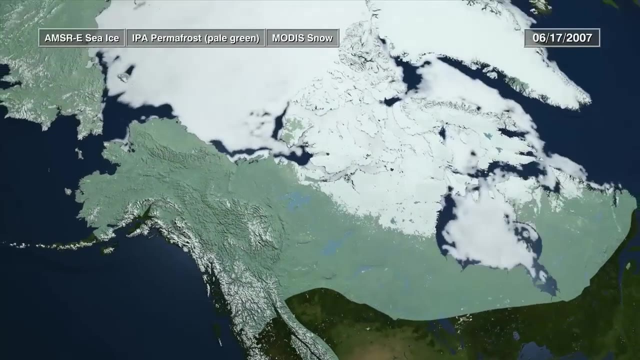 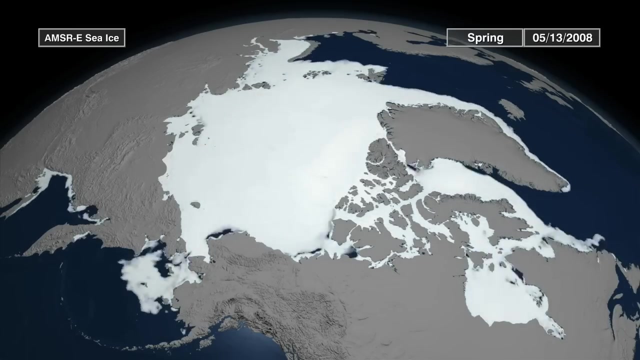 thaw. These regions are unusual in the mid-latitudes, but farther north permafrost is more widespread and continuous, covering nearly a fifth of the land surface in the northern hemisphere. Sea ice varies from season to season and from year to year. 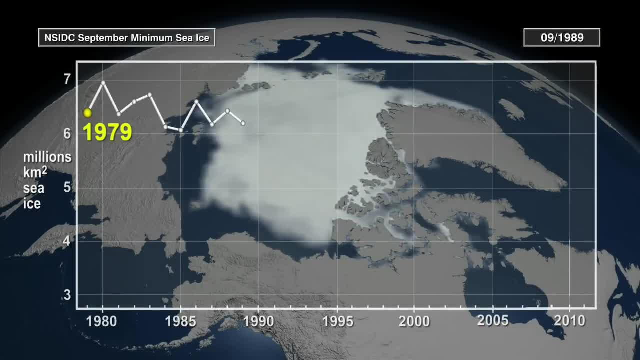 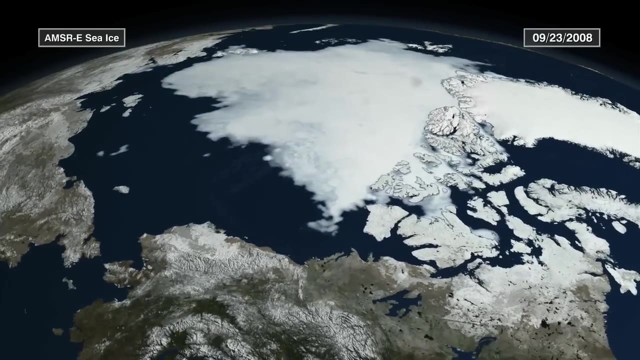 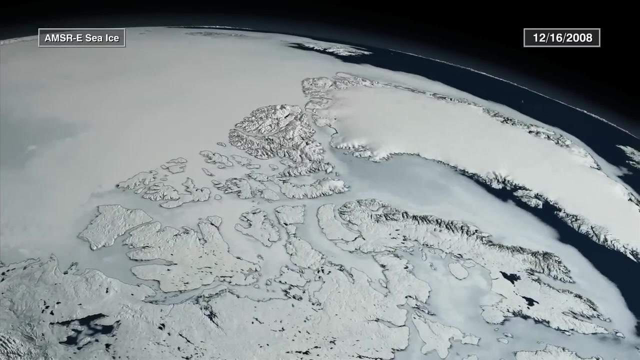 Data show that Arctic sea ice has shrunk dramatically in the last few decades. The effects could be profound. As polar ice decreases, more open water could promote greater heating. More heating could lead to faster melting, reinforcing the cycle. If this trend continues, the Arctic Ocean could be ice-free in the summer by the end. 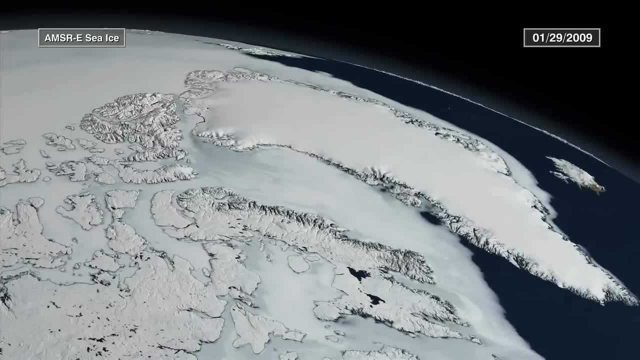 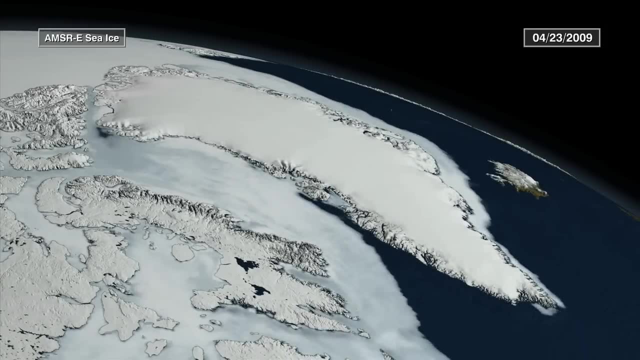 of the century. These changes in ice cover are not limited to oceans. Greenland's ice sheet contains nearly a hundred ice sheets. The Arctic Ocean is the largest ice sheet in the world. It covers nearly 10 percent of the Earth's glacial ice. 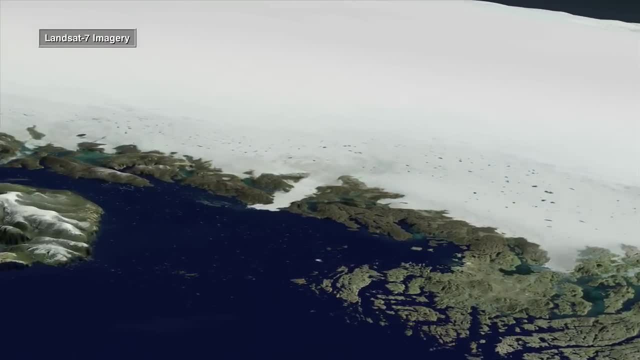 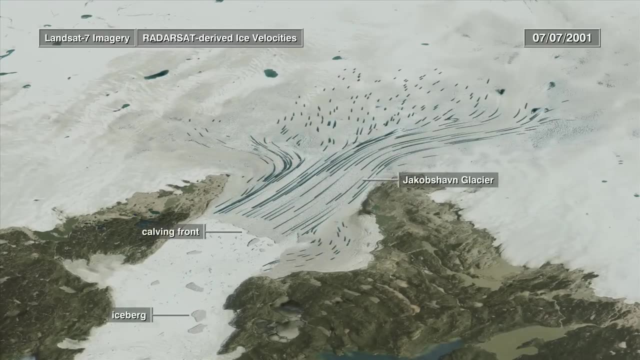 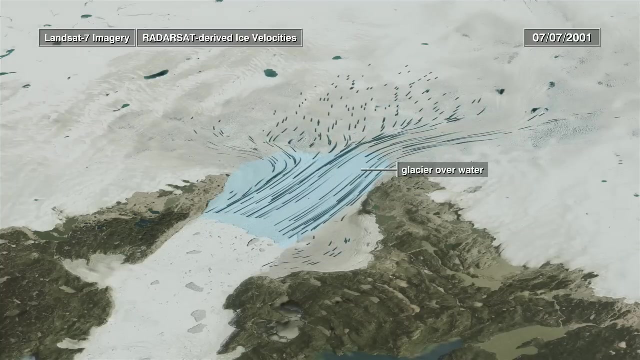 Glaciers in western Greenland produce most of the icebergs in the North Atlantic. After decades of stability, Greenland's Jakobshavn ice stream, one of the fastest-flowing glaciers in the world, has changed dramatically. The ice has thinned and the front retreated significantly. 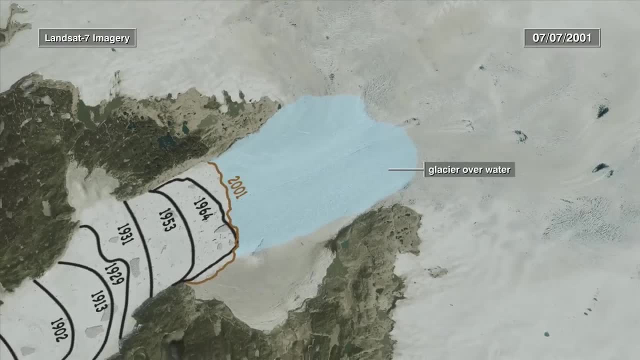 Between 1997 and 2003, the glacier's flow rate nearly doubled. The ice has been thinned and the front retreated significantly. Between 1997 and 2003,, the glacier's flow rate nearly doubled. The ice has been thinned and the front retreated significantly. 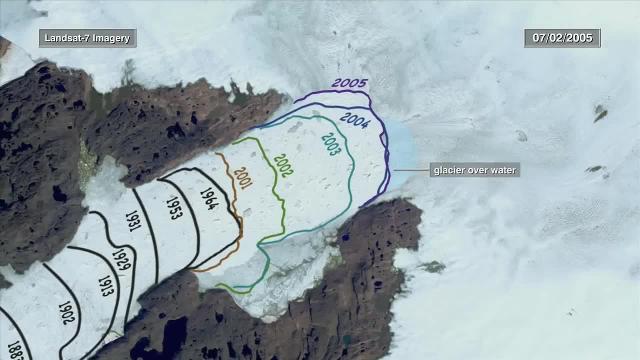 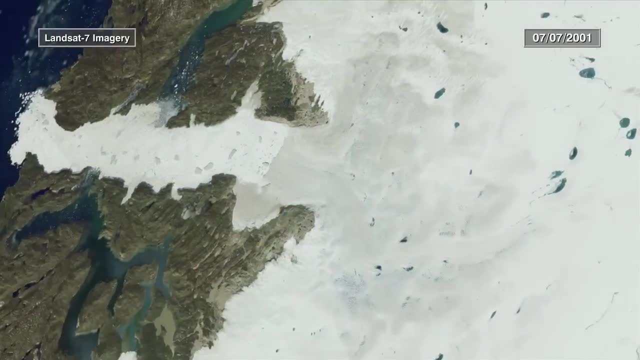 More and more glaciers have been raised up and caught on the surface. Fromذary ice autocorrosions have affected about five hundred. laters Theji and more weight snow front and pressure offered by the ice, and bothの zeigen the tavaí green. 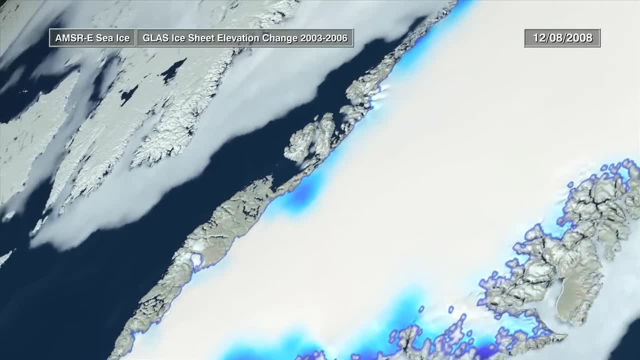 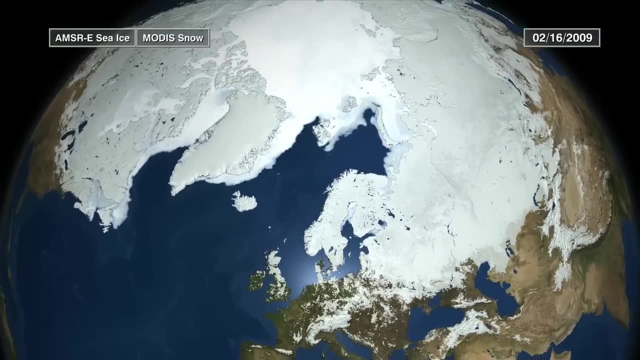 Theleri of snow have fundamentally lost more activity than other glaciers. concrete changes were made resulting inrint ofнем height increases. Several years after the Earth hit, the Arctic Ocean ge pokemon erupted, meaning that most lunar ecosystemsmy world behavior hadatter as an afterglow of the Earth.